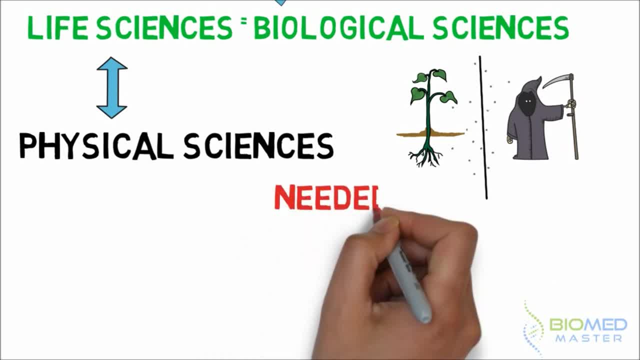 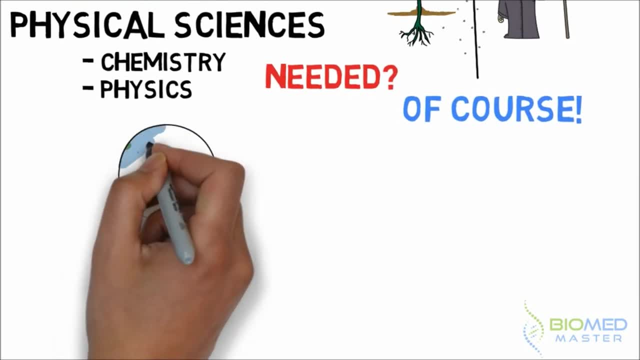 Now, does this mean you don't need to know anything about physical sciences if you want to become a biomedical scientist? Wrong, Of course. you need the basics of chemistry and physics to build upon in your further studies. After all, life wouldn't exist if there wasn't a physical earth with soil, metals, minerals, oceans and atmosphere. right? 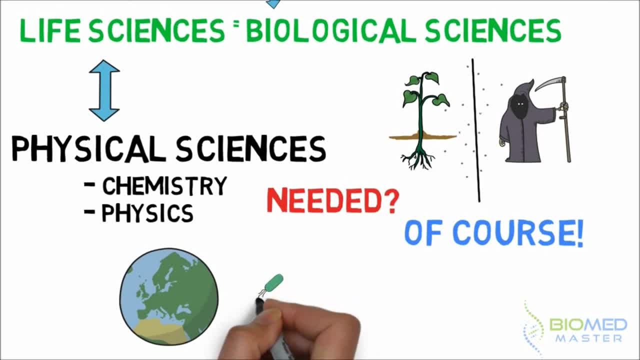 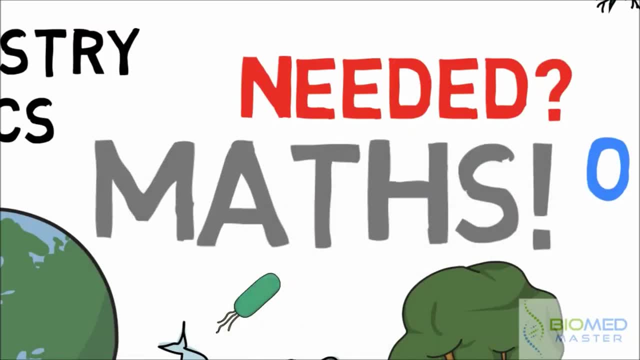 So as life needed these foundations of physical stuff to thrive upon, so will you need the fundamentals of physical science to progress in biomedical sciences. Oh, and also, don't forget, you will need some mathematics too. The second part, medical, obviously refers to medicine. 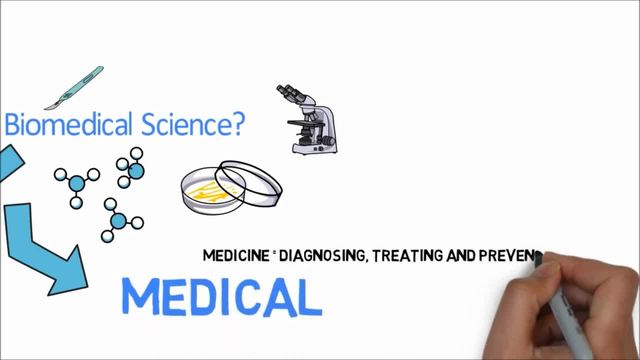 Duh Medicine is defined as the science or practice of diagnosing, treating and preventing disease, typically what doctors do, And by doctors I mean clinicians, those with the stethoscopes, not the PhDs, those with the pipettes. 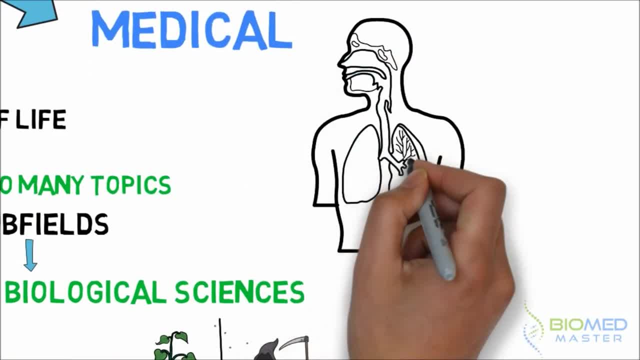 So, basically, if you want to do biomedical science, you need a big interest in biology and medicine. Well, here's something important which you can directly tell from the name itself. So, coming back to me saying earlier that biology is a broad term, well, here's where biomedical science narrows down. 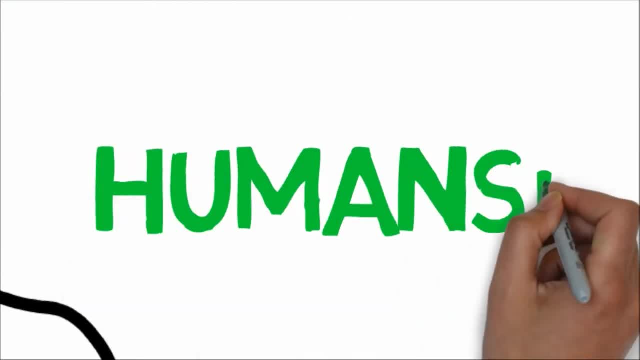 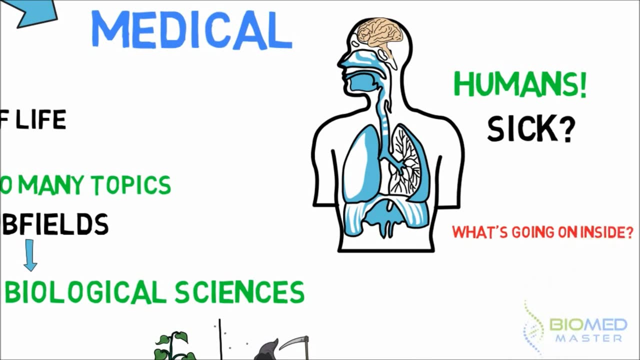 We're only interested in the human being. The medicine part of it means you should be interested in how human biology functions in health, and this functions in disease. but rather than treating patients as doctors, do we typically want to expand the knowledge on the mechanisms underlying human diseases? 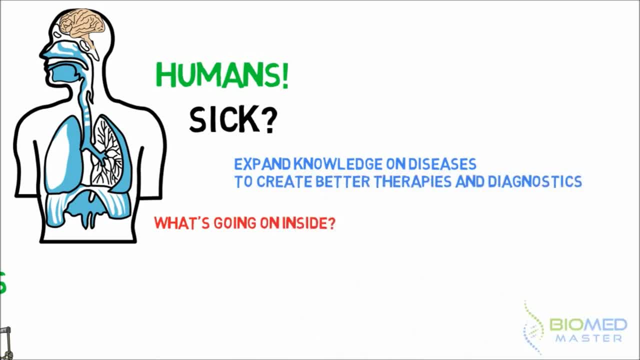 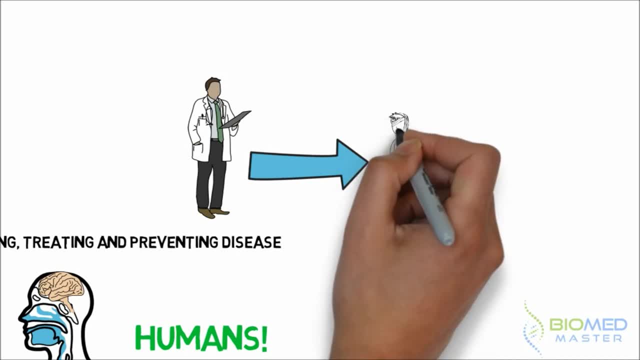 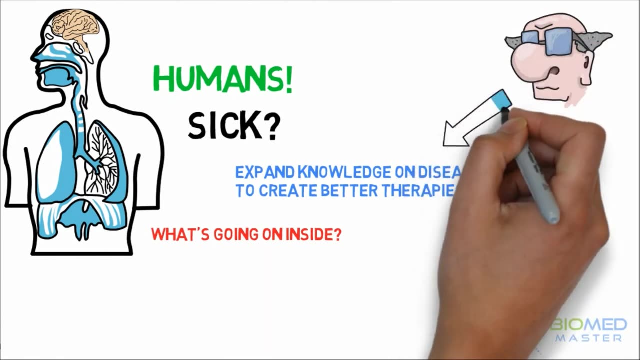 in order to come up with better drugs, therapies or diagnostics. So where the clinicians focus on treating the patients the best, the best way they can with the tools that are already there, we, as biomedical scientists, try to find better ways to treat patients or even lay foundations for finding a drug for a disease which was untreatable before. 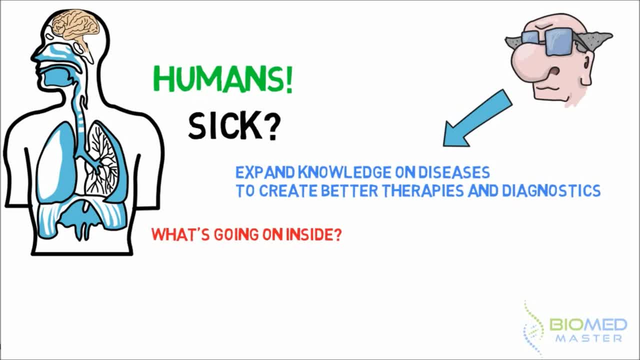 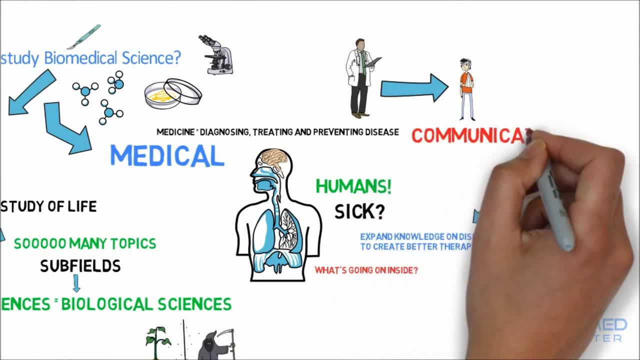 So, in essence, we do the research to make sure clinicians can focus their time on treating the patients, But we also, of course, need the medical lingo for us to communicate about our research findings to those clinicians. Now you might be wondering about all those other bio-something majors like biochemistry. 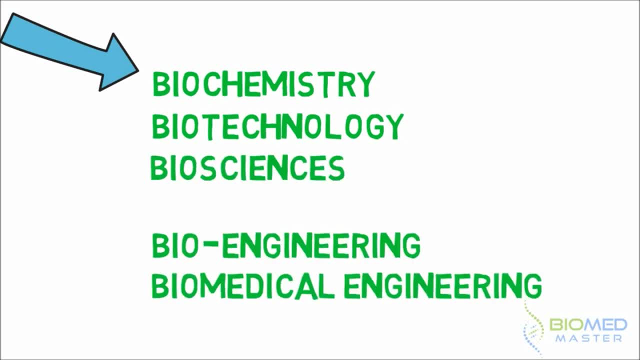 biotechnology, biosciences, bioengineering, biomedical engineering. Well here's the thing: there's a lot of overlap between these majors, but the difference is on the more in-depth focus. So obviously the engineering majors are more focused on building stuff by studying more engineering subjects.